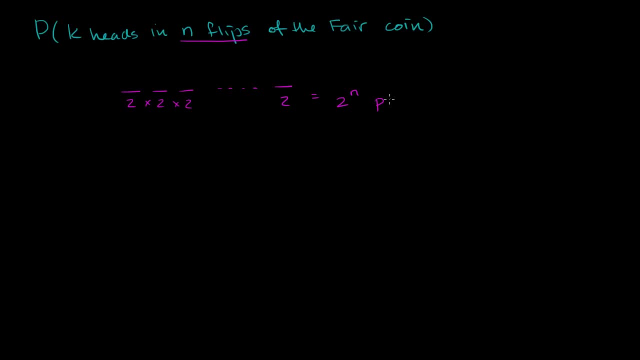 This is going to be equal to two to the nth possibilities. Now let's think about how many of those equally likely. these are all equally likely possibilities. this is a fair coin. Let's think about how many of those equally likely possibilities involve k heads. 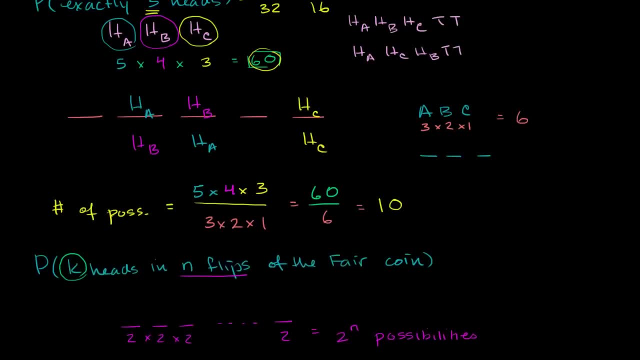 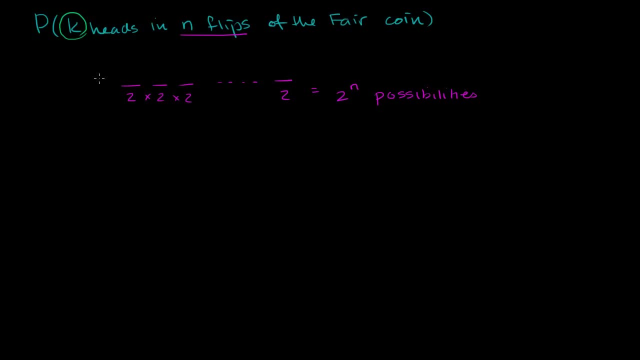 Well, just like we did for the case where we had, where we're thinking about three heads, we thought, think about three heads. We say, well, look, the first of those k heads, the first of those k heads, how many different buckets could it fall into? 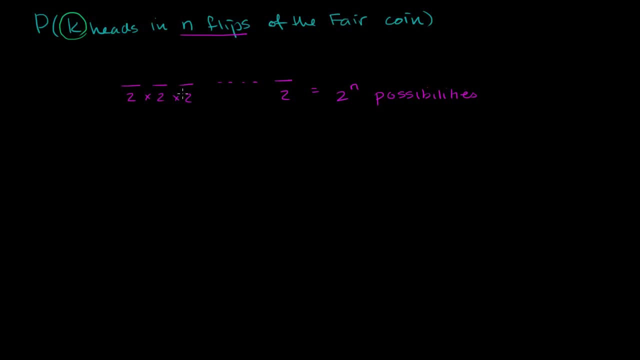 Well, the first of the k heads could fall into n different buckets, right, It could be the first flip, second flip, all the way to the nth flip, Then the second of those k heads- and we don't know exactly how many k is- 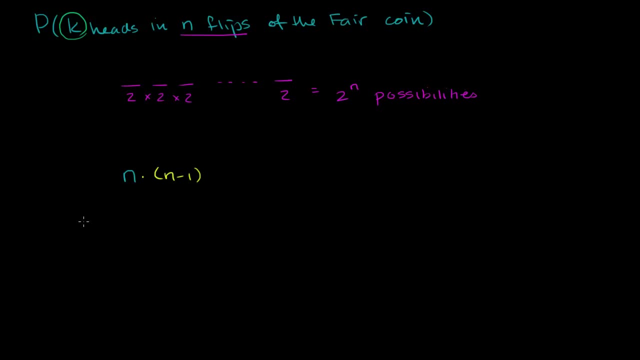 will have n minus one possibilities, n minus one possibilities, And then the third of those k heads will have n minus two possibilities, since two of the spots are already taken up, And we would do this until we have essentially accounted for all of the k heads. 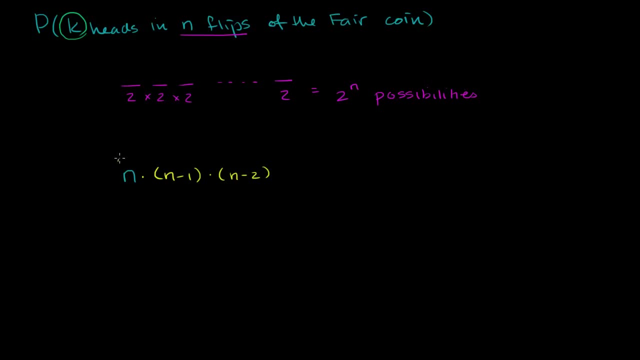 So this will go down all the way to. so this, we will multiply. the number of things we're multiplying is going to be k One for each of the k heads. So this is one, two, three, and then you're going to go to all the way to n. 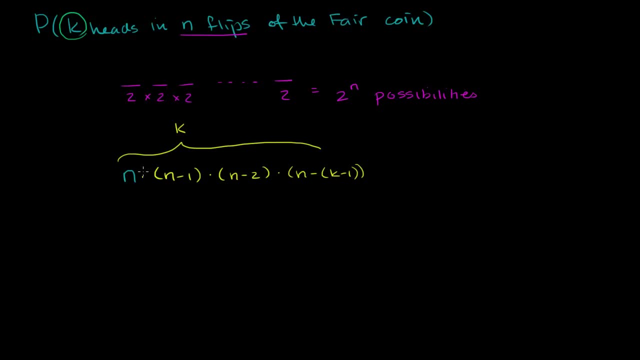 minus k, minus one, And you could try this out in the case of five. When n was five and k was three, this resulted in five times, four times, and actually we just had to go times three, and actually that was this term right over here. 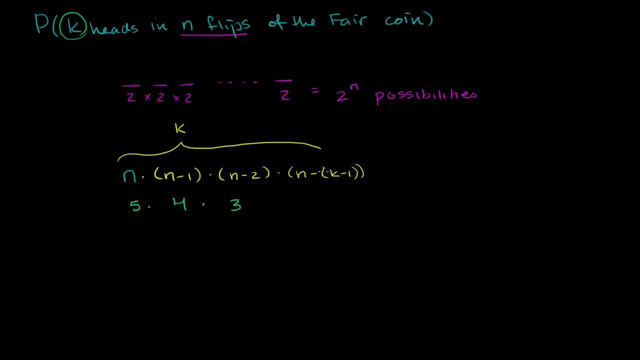 So I'm doing a case that is a little bit longer, where k is a slightly larger number, because this right over here is five minus two. That is this one over here. So let me actually let me, just so not to confuse, let me write it like this: 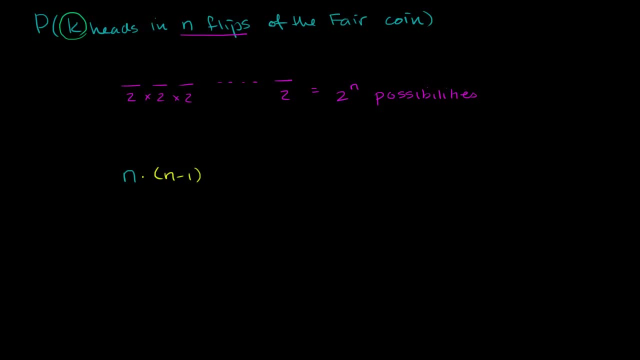 Let me write it like this: So you'll have n spots for that first head, n minus one spots for that second head, And then you keep going and you're going to have a total of these k things you're multiplying And that last one is going to be is going to have n minus n minus k minus one possibilities. 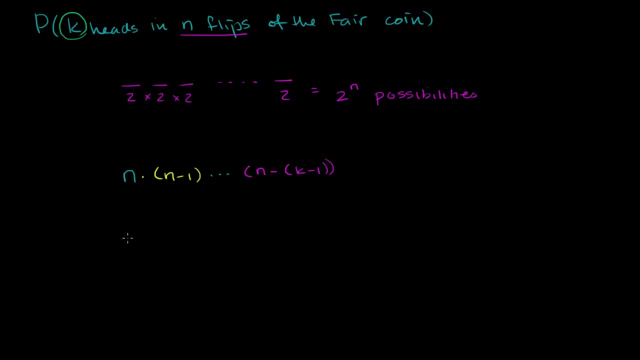 And now hopefully it'll map a little bit better to the one where we had five flips and three heads, Because here there was five possibilities for the first head, four possibilities for the second head, and then n is five, five minus two. you had three possibilities for the last head. 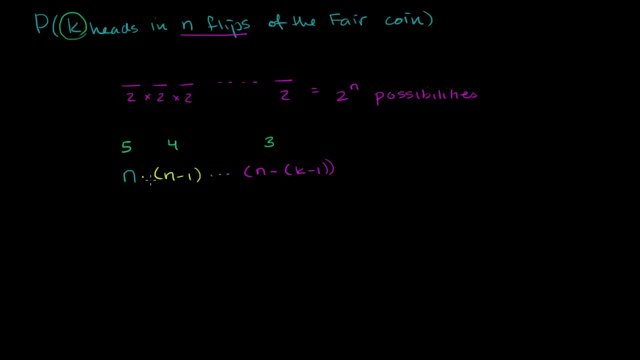 So this actually works. This is the number of spots where, or the number of ways that we could put, that we can stick those heads in those or that we can stick. we can put three heads into five different possible buckets. Now, just like the last video, we don't want to over count things because we don't care about. 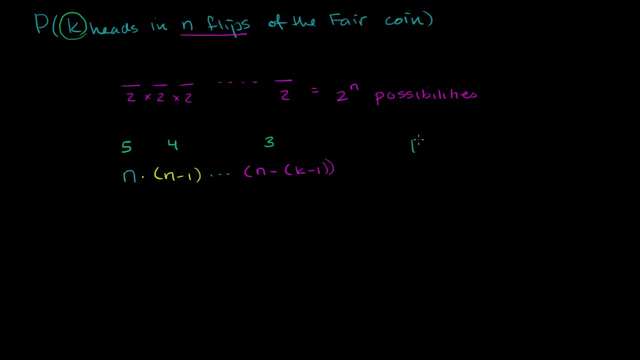 about the order. We don't want to differentiate. we don't want to differentiate, we don't want to differentiate one ordering of heads, And I'm just going to use these letters to differentiate the different heads. We don't want to differentiate this from this. 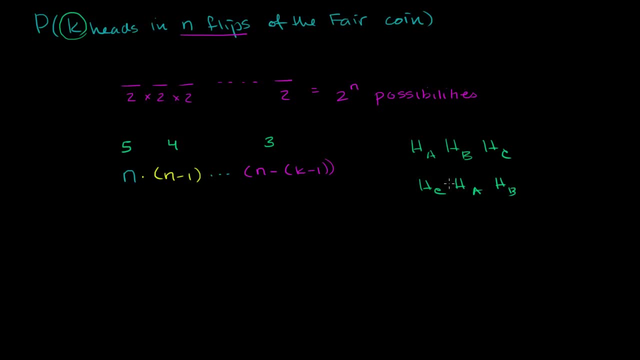 Heads A, heads B or any of the other orderings of this. So what we need to do is we need to divide this. we need to divide this number so that we don't count all of those different orderings. We need to divide this by the different ways that you can order k things. 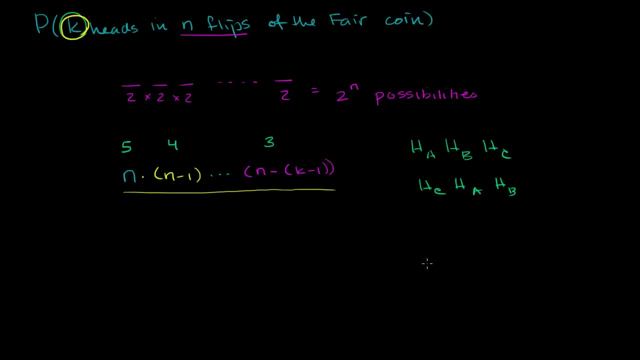 The different ways that you can order k things. So if you have k things, so you know one thing, two things, all the way to k things, how many ways can you order it? Well, the first thing can be in k different positions. 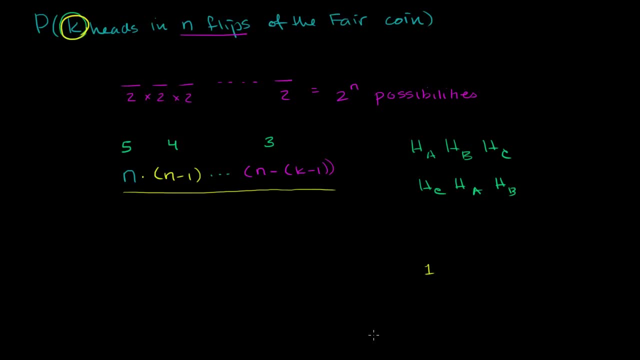 K different positions. Or maybe I'll do it like this, Maybe I'll, I'll. I'll do it thing one, I'll call it T for thing Thing one, thing two, thing, three, all the way to thing k. 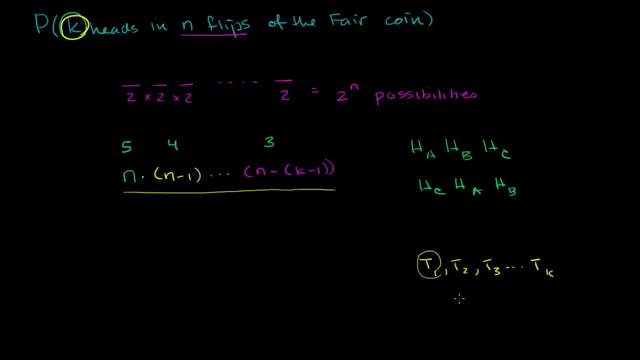 How many different ways can you order it? Well, thing one can be in k different ways, K different positions, Then k thing two will be in k minus one positions, And then all the way down to the last. one is only going to have one position. 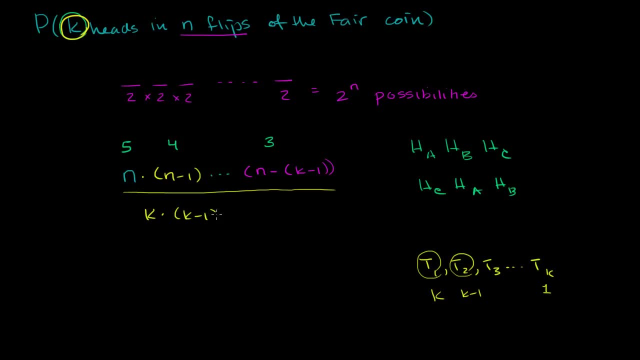 So this is going to be k times k minus one times k minus two, all the way down, all the way down to one. And in the example where we had three heads in five flips, this was three times two, all the way down to one. 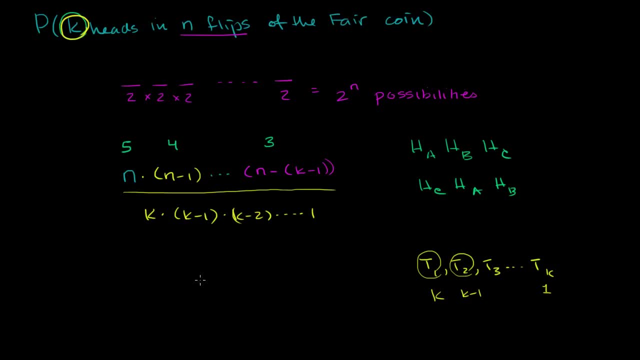 Three times, two times one, And so is there a simpler way that we can write this? Well, this expression right over here, this expression right over here, this is the same thing as k, factorial, And if you haven't ever heard of what a factorial is, 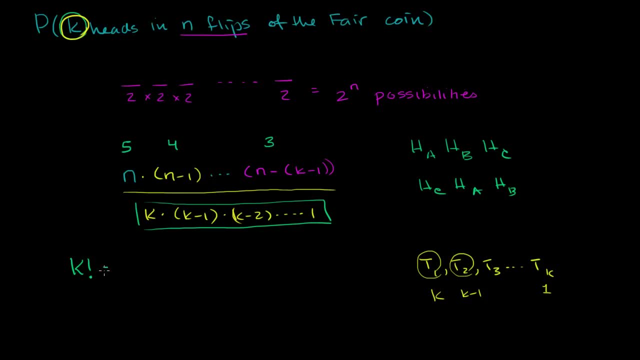 it's exactly this thing right over here. K factorial literally means k times k minus one times k minus two, k minus two, all the way down to one. So, for example, two factorial is equal to two times one. Three factorial is equal to three times two times one. 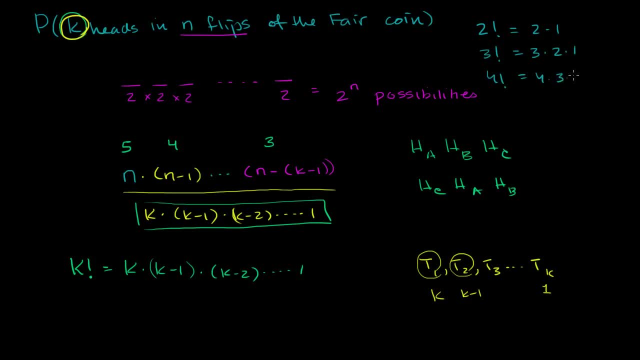 Four factorial is equal to four times three times two times one. So- and it's actually a fun thing to play with- Factorials get large very, very, very, very fast. So anyway, this denominator right over here can be rewritten as k factorial. 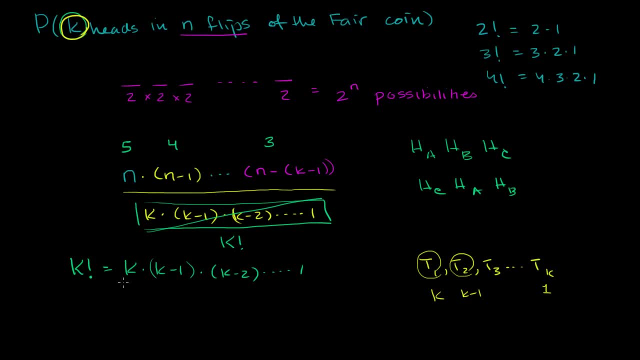 This right over here can be rewritten as k- factorial, And is there any way to rewrite this numerator in terms of factorials? So if we wrote, if we were to write n factorial, so let me see how we can write this: If we were to write n factorial, get some real estate over here. 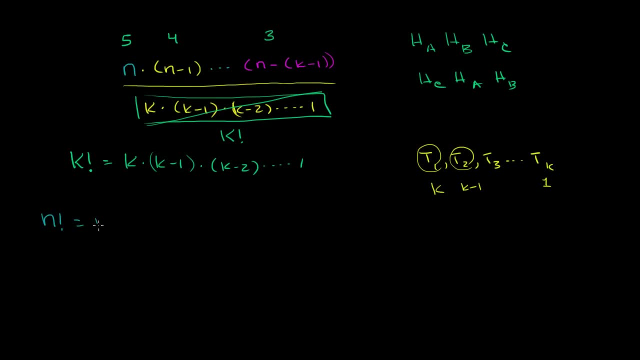 So n factorial would be equal to n times n minus one times n minus two, all the way down, all the way down to one, All the way down to one. That's kind of what we want. We just want the first k terms of it. 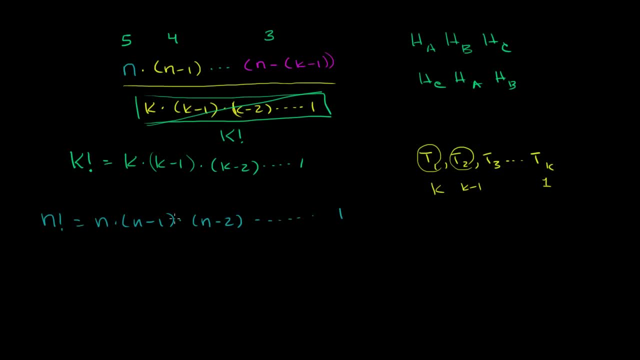 We just want the first k terms of it. So what if we divide this by: so let's divide this by n minus k factorial, So n minus k K factorial. So let's think about what that is going to do That if we have n minus k factorial, that is the same thing as 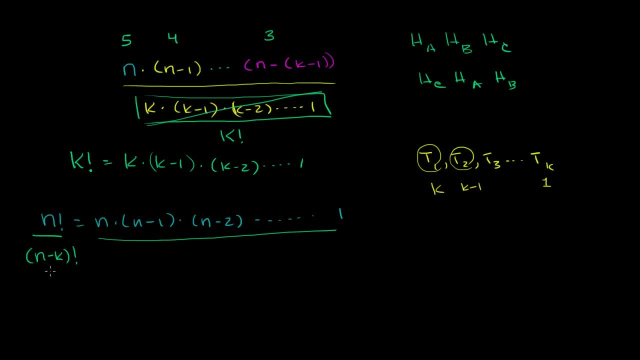 we have to do a little bit of algebraic manipulation right over here. That is the same thing as n minus k, n minus k times n minus k minus one, n minus k minus one minus one. So n minus k factorial is going to be n times n minus k, times n minus k minus two. 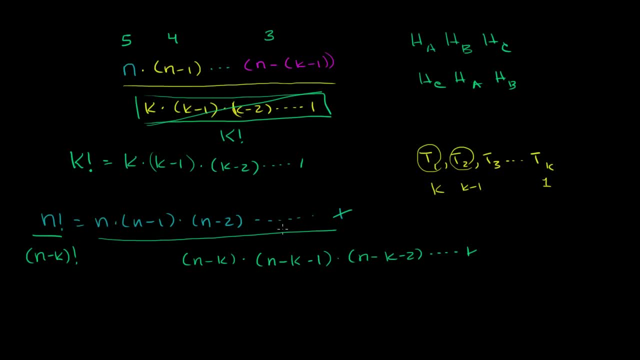 all the way down to one, And what I want to: when you divide these, the ones going to cancel out And what you may or may not realize and you can work out the math- is: everything is going to cancel out here until you're just left with up here. 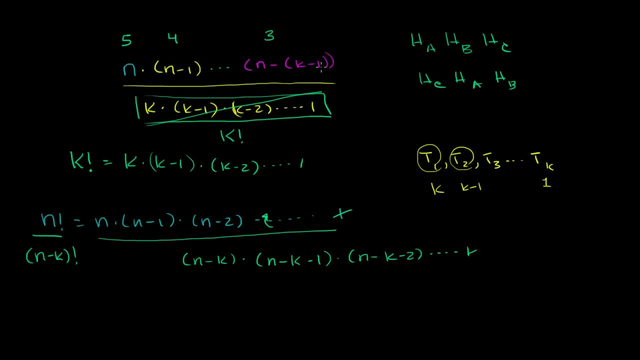 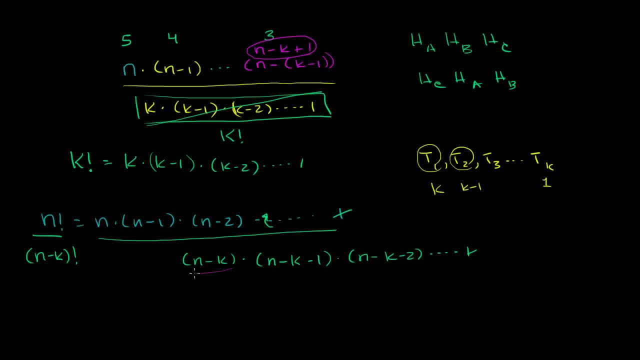 So n minus k plus one is the integer. that's one larger than this right over here. So if you were to divide it out, this would cancel with something up here. this would cancel with something up here. this would cancel with something up here. 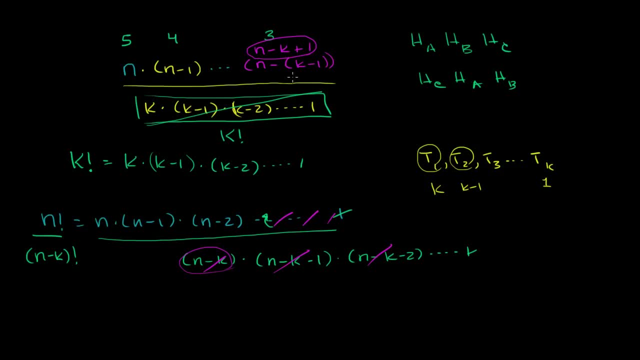 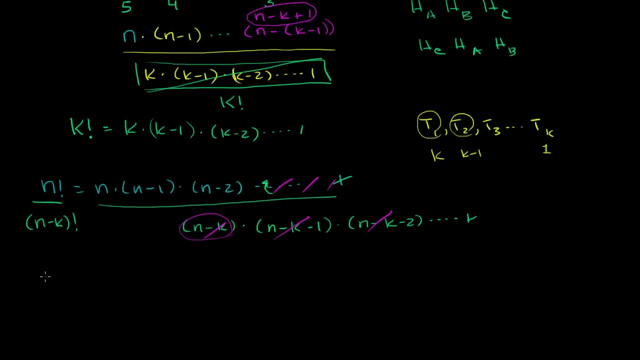 And what you're going to be left with is exactly this thing over here, And if you don't believe me, if you don't believe me, we can actually try it out. So let's think about what five factorial, what five factorial over five factorial is. 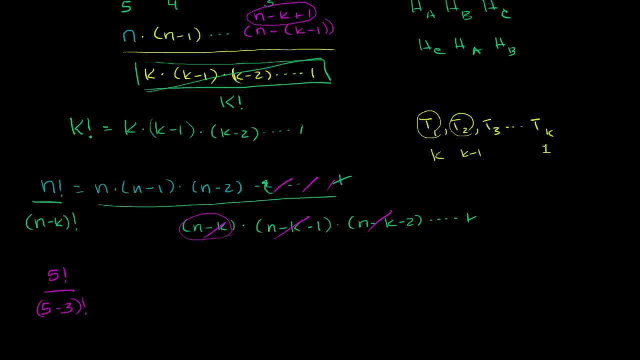 Five minus three factorial is going to be over five minus three factorial. So this is going to be five times four times three times two times one. So all of that stuff up there all all the way down to one Over five minus three is two over two factorial two times one. 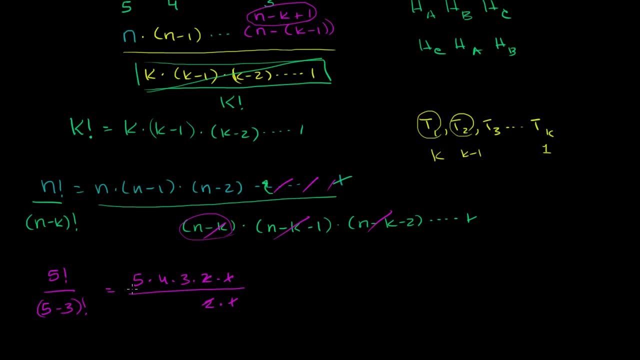 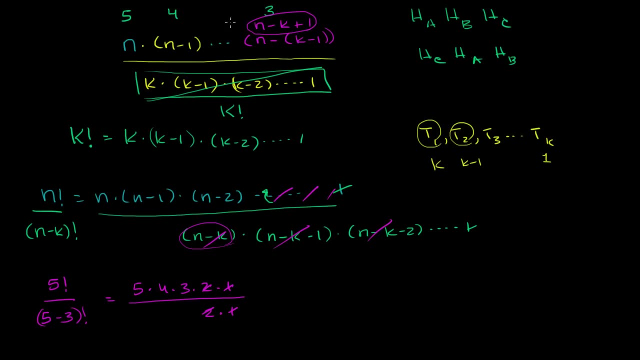 Two cancels with two, one cancels with one. you don't even have to worry about that and you're just left with five times four times three, Exactly what we had up here: five times five times four times three. And so, in general, if you wanted to figure out the number of ways to stick, two things. 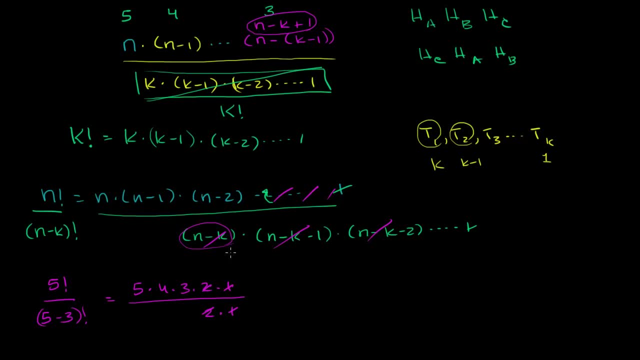 in five chairs and you don't care about differentiating between those two things. you're going to have this expression. you're going to have. you're going to have this expression right over here, which is the same thing as this, right over here. 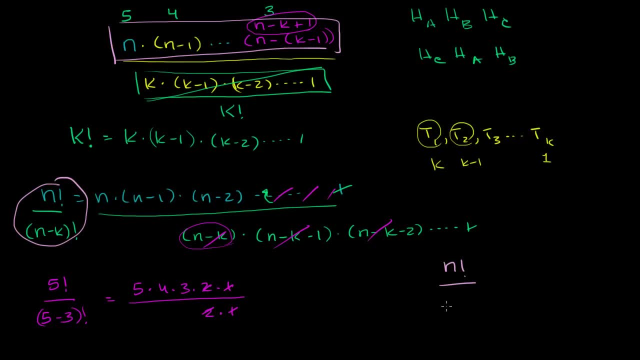 So you're going to have n factorial over n minus k factorial and then you're going to divide it by this expression right over here, which we already said is the same thing as k factorial. So you're also going to divide it by k factorial. 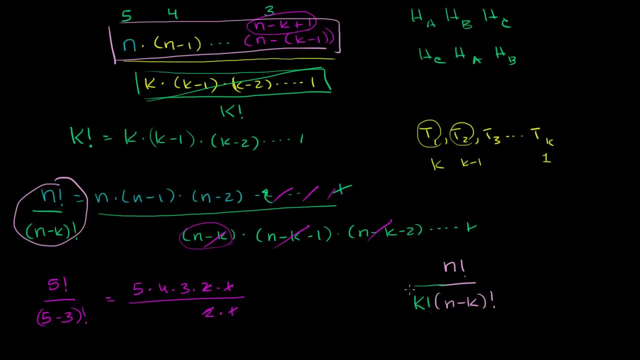 And then you have a generalized way of figuring out the number of ways you can stick two things, or the number of ways, actually I should say the number of ways you can stick k things in n different buckets, k heads in n different flips. 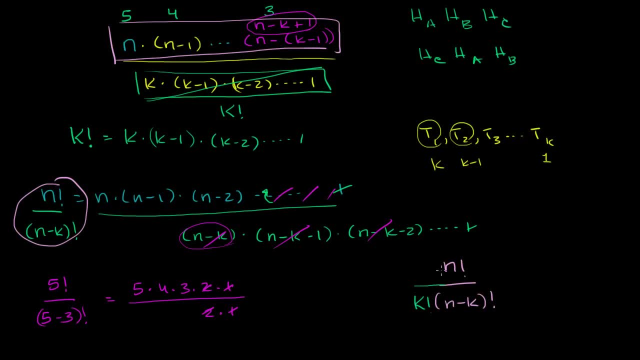 And so another way of writing it. And this is actually a generalized formula for binomial coefficients. So another way to write this is the number of ways, given that you have n buckets, you can put k things in them without having to differentiate it. 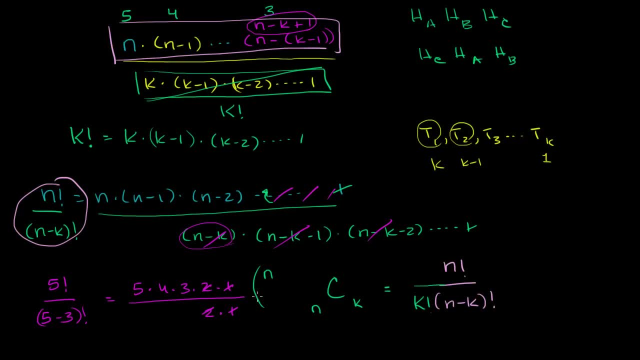 Or another way to think about it is if you have n buckets or n flips and you want to choose k of them to be heads, or you want to choose k of them in some way, but you don't want to differentiate. 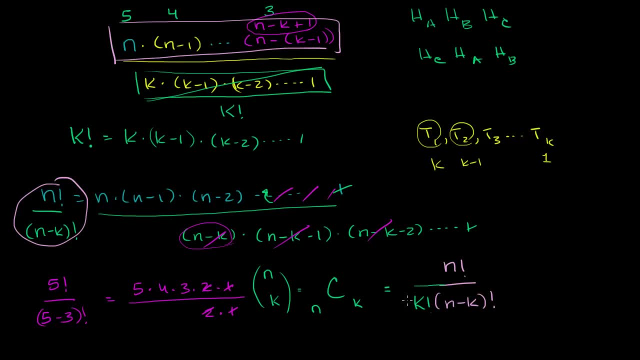 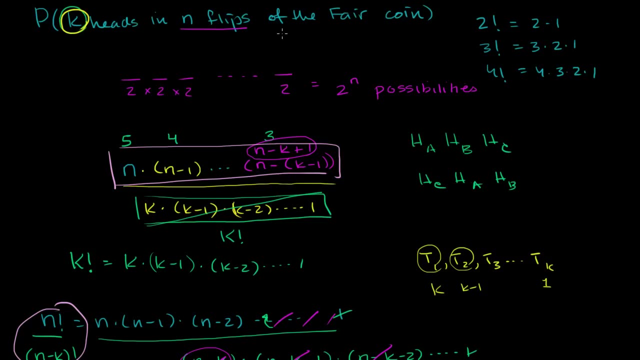 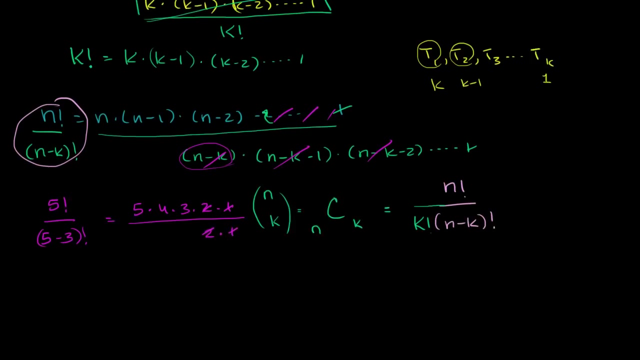 So all of these are generalized ways for binomial coefficients. So, going back to the original problem, what is the probability of getting k heads and n flips of the fair coin? Well, there's 2 to the n equally likely possibilities. So let's write this down. 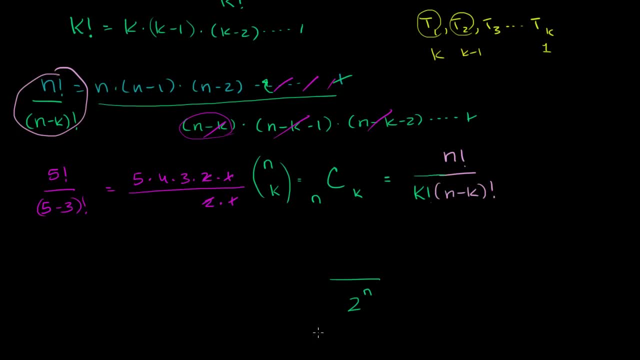 So the probability of 2 to the n equally likely possibilities, And how many of those possibilities result in exactly k heads? Well, we just figured that out during this video. That's the number of possibilities. So n factorial over k heads, k factorial times, n minus k factorial. 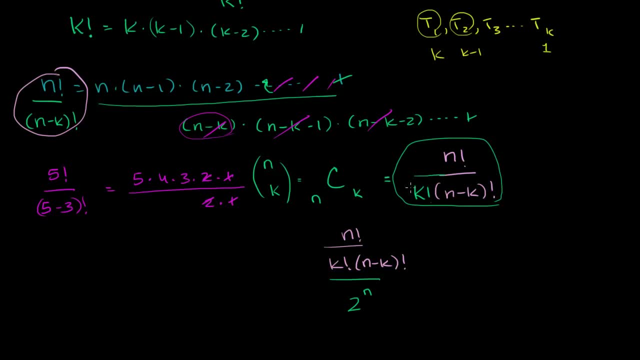 Now it probably is an OK idea to memorize this, But I'll just tell you frankly, the only reason why I still know how to do this, 20 years after first seeing it, or whenever I first saw it, is that I actually 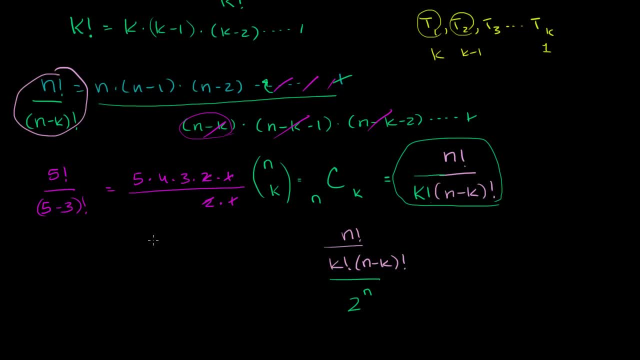 just like to reason through it every time. I like to just reason through. OK, I've got 5 flips. 3 of them need to be heads. The first of those heads can be in 5 different buckets and the next in 4 different buckets. 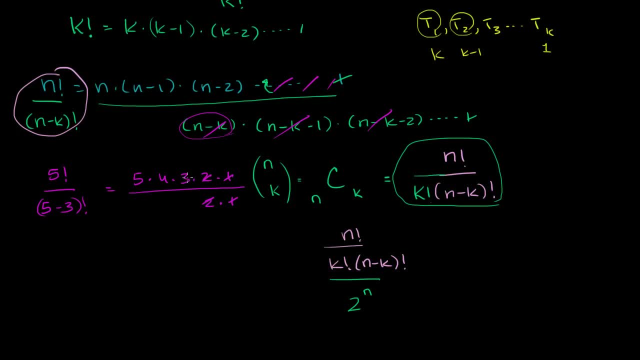 and the next one in 3 different buckets. And then, of course, I don't want to differentiate between all of the different ways that I can rearrange 3 different things, So I have to make sure that I divide it by 3. factorial: 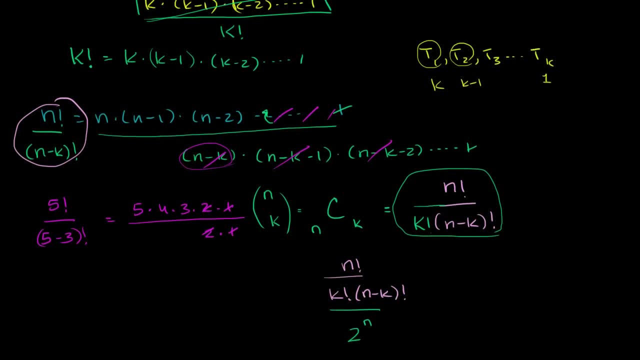 by 3 times, 2 times 1.. I want to make sure that I divide it by all of the different ways that I can arrange 3 different things.